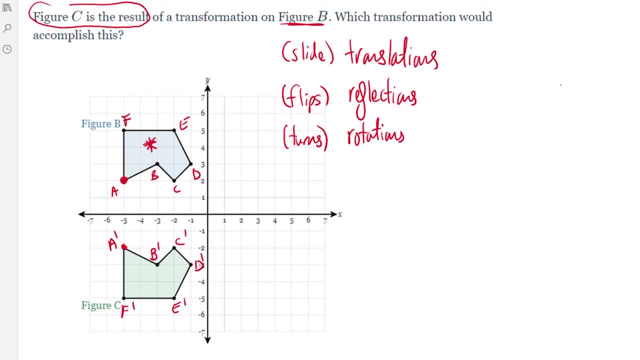 E, prime, F, prime. Okay, So I wanna show you something. This only happens with a reflection. Remember, a while ago I was telling you guys, if you look into a mirror and you look at your reflection and, let's say, you're wearing a t-shirt and it has a word, 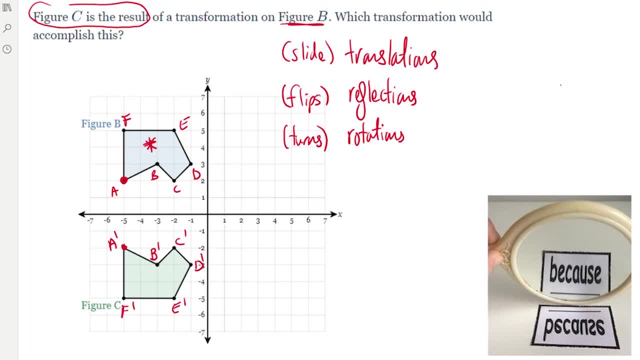 on it. when you look into the mirror, you're gonna see that the word looks different, right? Not not backwards necessarily, but the letters are flipped, Like the letter E would be facing the wrong way. Certain, you know, different letters will be facing in the wrong direction. 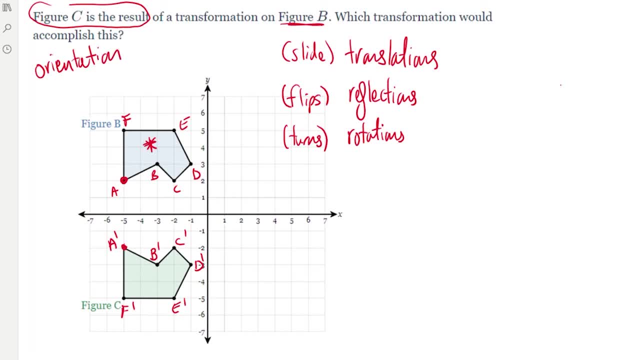 We call that orientation, and the orientation changes with a reflection. It's the only one where the orientation changes. Notice that in the in figure B, if we're reading A, B, C, D, E, F, we're going in that direction, right Like you have to read around the shape and that direction. 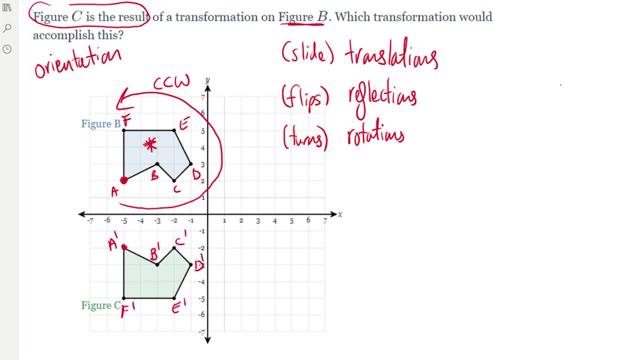 is a counterclockwise direction. It's the opposite direction of how a clock turns. But if you look at the resulting image, well, it goes A, B, C, D, E, F, It it turns in the other. 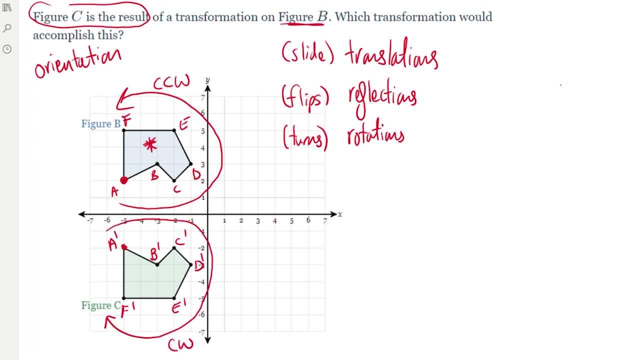 way right. This is a clockwise direction when you're reading around the shape. So that's, that's one way to verify that you actually have a reflection. The only problem is if you do two reflections. let's say, I reflected this shape to this and then I took the shape and I reflected. 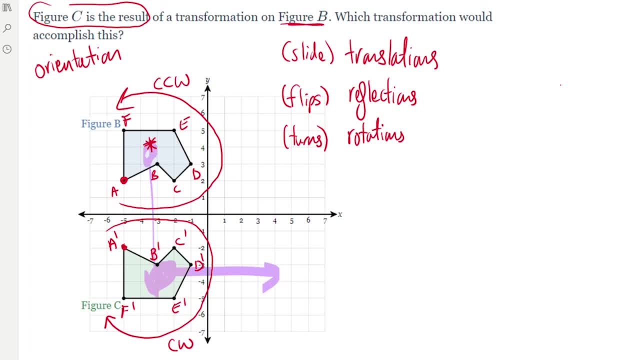 it over here, Then the orientation is going to change back to the original orientation. Last thing you need to do is, when you say reflection, you have to say a couple other things as well. You have to say, actually, just one other thing You have to say across. 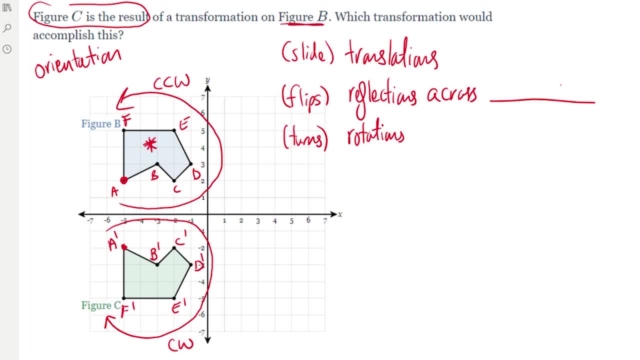 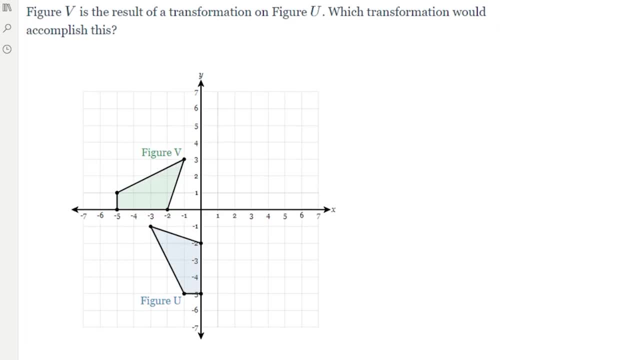 and you have to say what line are you reflecting across. And in this case it's just the X axis. Figure V is the result of a transformation of figure U. So figure V is a result, That means figure U is the original one. I'm just going to put a star. 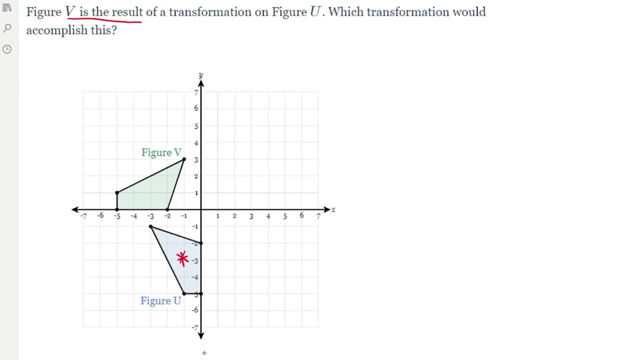 Anytime you see a star in a shape, that means that that's the original one. Can it be a reflection? Let's say I were to read the shape. Let's say: that's A and I'm going, I'm going to slope downward here. That's B, that's C, that's D. Now I know this is my A prime.